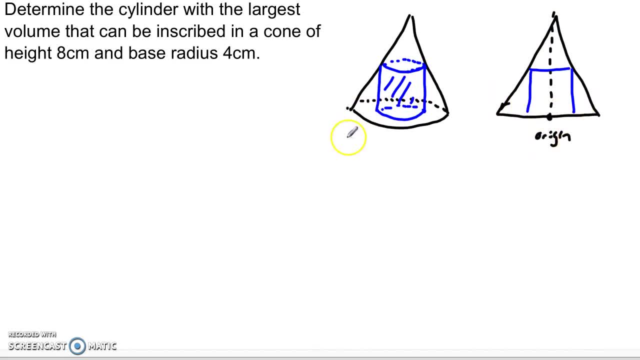 let this be the x-axis, then we can define everything pretty easily. So what are some of the things that we're going to need to do to make this work? Well, these are the variables we have to control, for here We've got to pay attention to r. 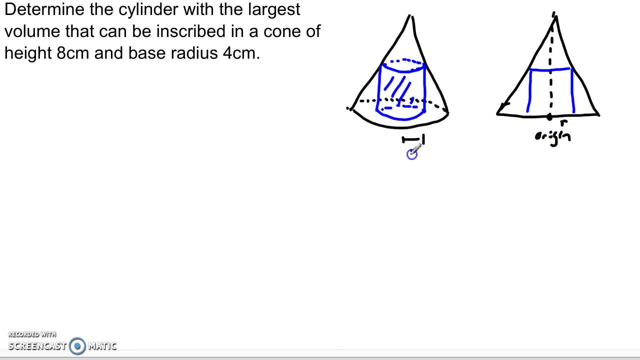 which is the radius of this cylinder. right, I want to pay attention to r, But I also need to pay attention to the height of the cylinder. I'll call that h and you know that'll be the same in each drawing: h here height, h here height. I guess I'll go over here. 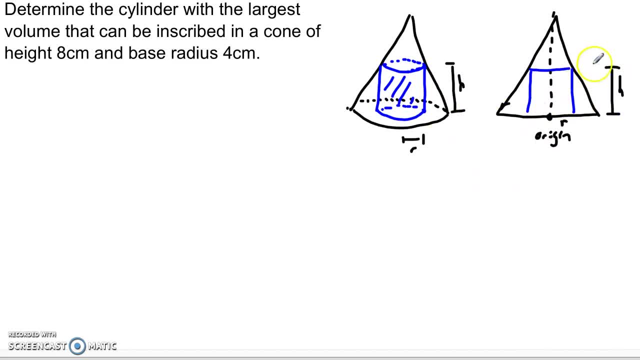 just put a little h right Now. how do I know that I need the radius and the height? Well, the volume of a cone, excuse me of a cylinder, is pi times the cylinder's radius, squared times the height of the cylinder. So in order for me to calculate this volume, I'm going 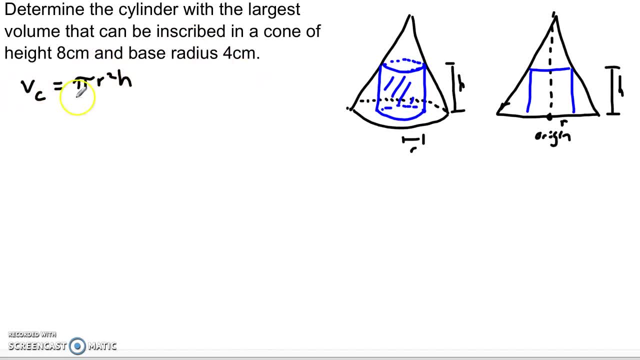 to need the radius, I'm going to need the height. Now that's two variables, and this comes up very often in these optimization problems. We have a function that we're looking to optimize with more than one variable. We need to get that down to one variable before. 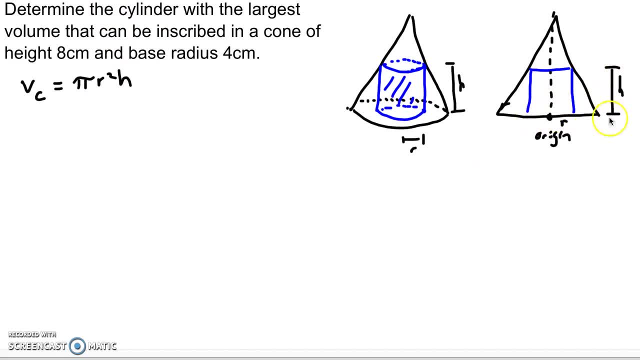 we can do anything. So we've got to figure out how the radius and the height are related to each other. Well, in this case that's a pretty simple relationship, Since my cone has a height of 8, that means that this up here is 8 on the right and this up here is. 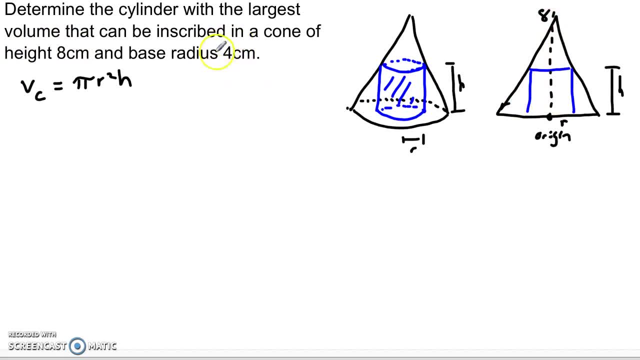 8 on the y-axis, or the height axis, if you will, And it has a radius of 4, that makes that this is 4 on the x-axis, or the radius axis, if you will. So this is actually just. 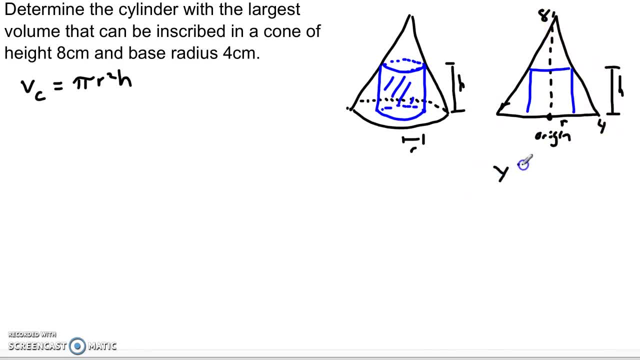 a linear equation, right? It's pretty simple to figure out. it's just: y equals 8 minus 2r, right? Excuse me, I shouldn't say y equals. I should say h equals, since this is height and radius. All right, so the height is equal to 8 minus 2r. it's simply a linear equation. 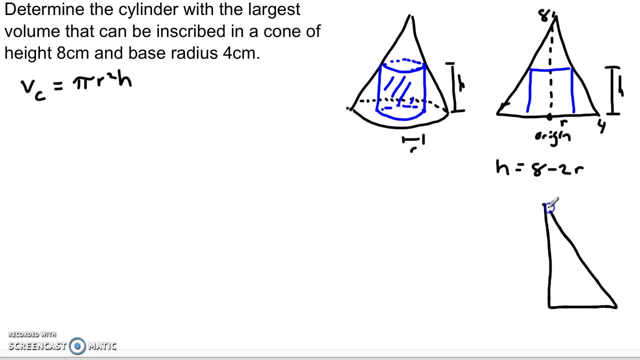 Something else that you can do- sometimes students find it easier to see this way- is you can think about similar triangles. So when I put the cone in here, there's actually two similar triangles. This is the cone in here. Well then, we know that this entire height is 8, and we know that this entire 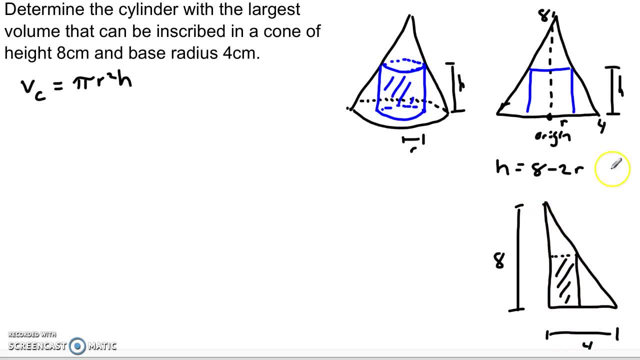 width is 4.. So in this large triangle we've got 8 by 4.. But then we can also think about just h, the height of my cylinder, which is right there, and just the radius of the cylinder is right there, which makes this part here 4.. 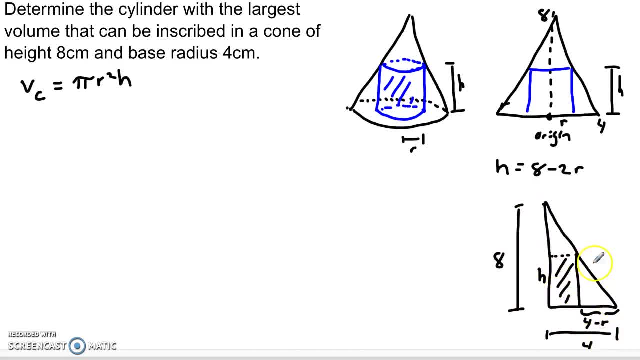 So we can say h over 4 minus the radius, And we can set up a proportion. These are similar triangles. We can say: 8 over 4 equals h over 4 minus r. right, That's coming from: 8 over 4 equals h, this height over 4 minus r. And then you know, 8 over 4 is just 2, so this: 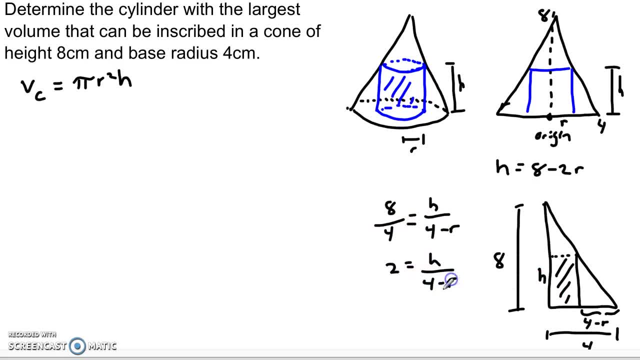 is 2 equals h over 4 minus r, which means 8 is, if we cross, multiply here, 8 minus 2r. Well, that is exactly the same thing as we had there. So it doesn't matter which way you set this up. whatever is more comfortable for you. What's important is that you have 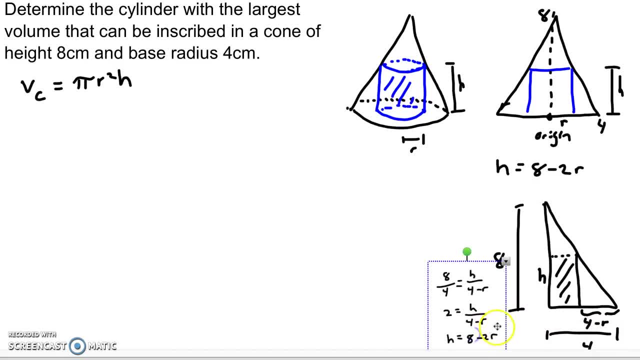 to figure out the relationship between those two variables so that you can eliminate one from the first equation. I'm just going to tuck that over there, so it's out of the way. I have a little bit more room, So back to my original formula here. Volume of the cone. 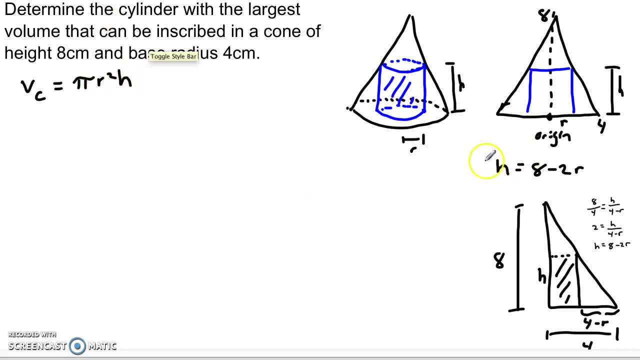 of the cylinder. rather is pi r squared h, But h is restricted right. h has to follow this relationship in this problem, So I can replace the h with that. I've got a formula for my volume of pi r squared times. 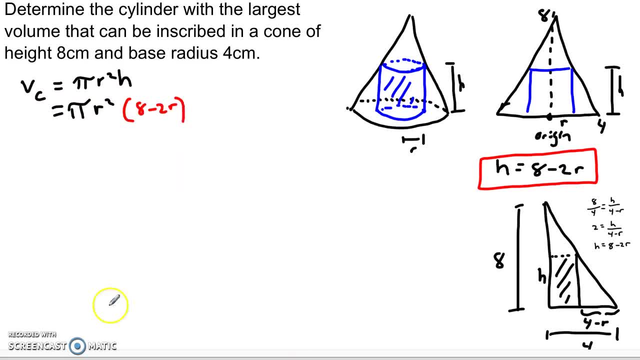 h, which is 8 minus 2r. Now we can of course, clean this up a little bit and we get the volume equal to, let's see, 8 pi r squared minus 2 pi r cubed. Now the good thing is. 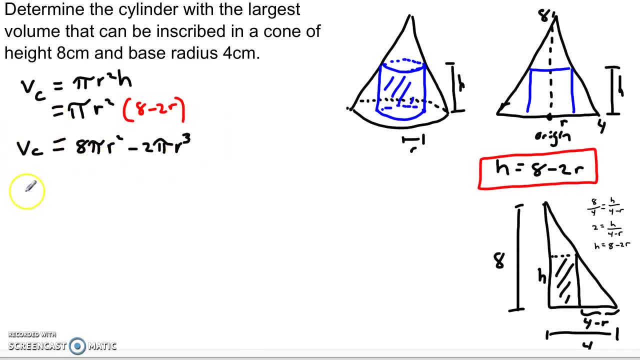 that this is again a nice polynomial function, so it's going to be really easy to work with. We're looking for, of course, the derivative, So this is just straight up power rule. again We have, let's see, 16 pi r minus 6 pi r squared. 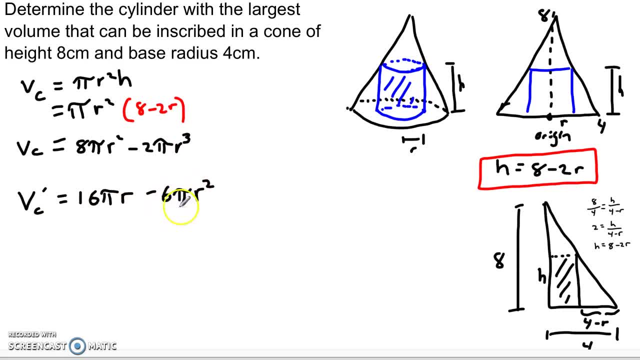 We can factor a little bit out of this. Let's see, we can pull out a pi and an r and at least a 2, it looks like. So let's go ahead and pull out a 2, pi, r, And then we'll get. 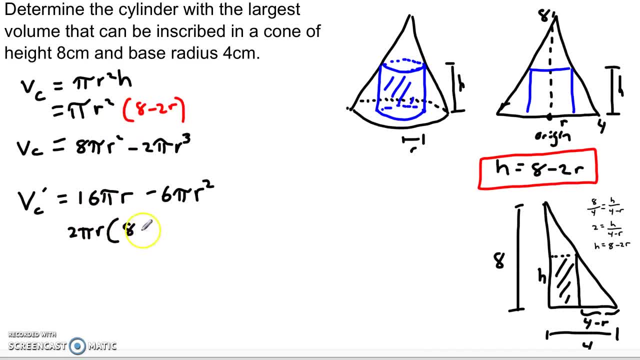 8. That'll give us 16 minus 3 r. If we go ahead and set that equal to 0, then we'll get two critical points, right. We get a critical point at r equals 0, which that's not really sensible, right? Because if the 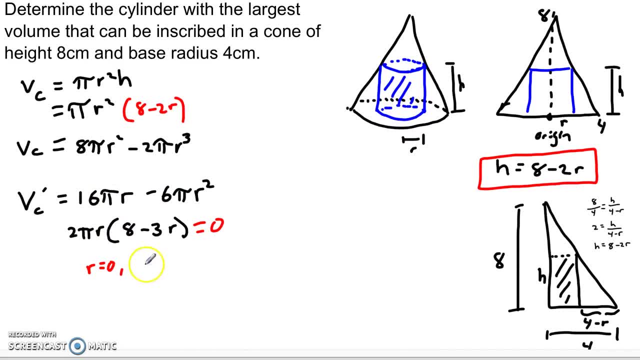 radius is 0, you have nothing going on there, so we don't have to worry about that one. We also get a critical point at r equals 8 thirds. So intuition should tell us that, of the two, this is going to be the point we're looking for. But again, let's keep good habits. 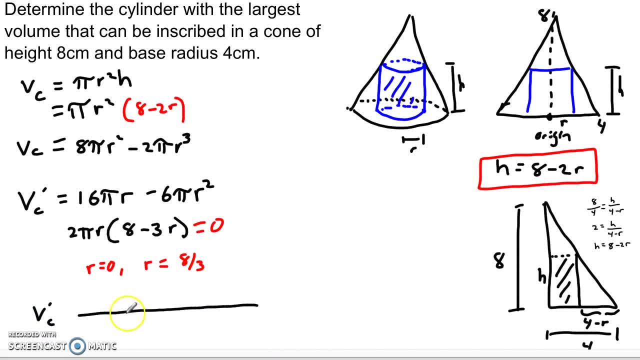 and let's write down the prime line. think about the analysis of the function and establish that it is in fact a relative max. So if I were to graph this parabola, it's going to look something like this: That tells: 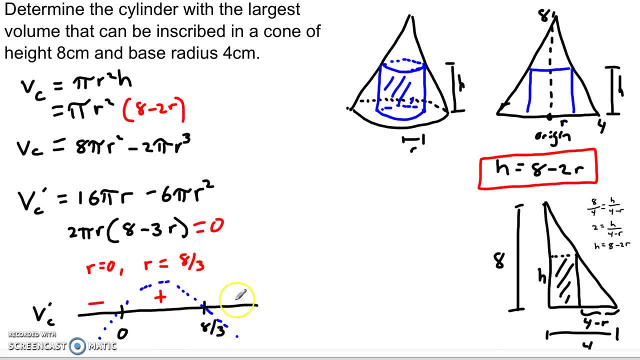 me that the sine of the derivative is negative up to 0,, is positive from 0 to 8 thirds and is negative from 8 thirds onward. So that tells me that this function, the original function, the volume function, is decreasing, then increasing, then decreasing. 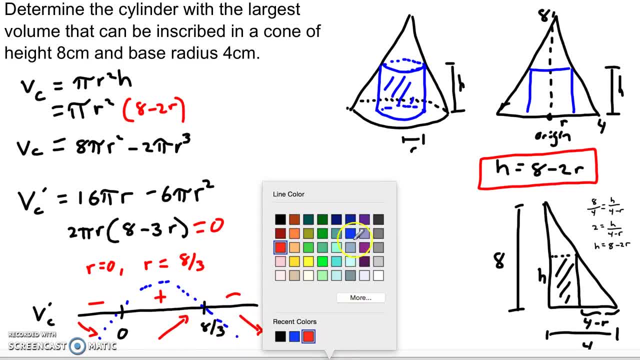 And that squares with our intuition, because of course, this tells us that we have a relative max point right here, maximum point here. So that's the point that we're looking for, the point where the radius is equal to 8 thirds. 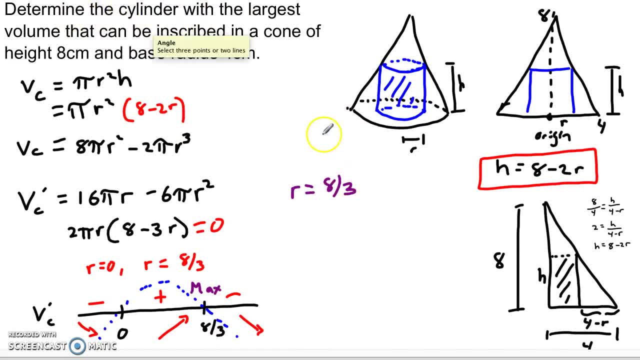 I believe that. let's see what is the answer. Determine the cylinder with the largest volume. So the radius is 8 thirds. We should figure out what the height is as well. We get that by simply plugging into there. So if the radius is 8 thirds, the height is 8 minus 2 times. 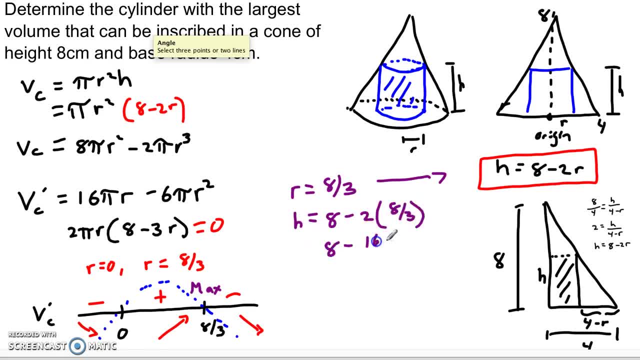 8 thirds, right, Which would be 8 minus 16 thirds. 8 is 24 thirds, so that gives us a height of 24 minus 16 thirds, or simply 8 thirds again. Aha, right, 16 up to 24, yeah, it's going to be. 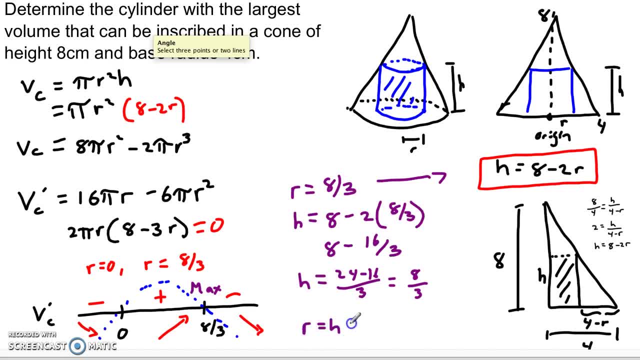 8 thirds. So we've got a radius equal to the height, which is equal to, in this case, 8 thirds. We have centimeters, or units in this case, so we'll go ahead and put centimeters down there. 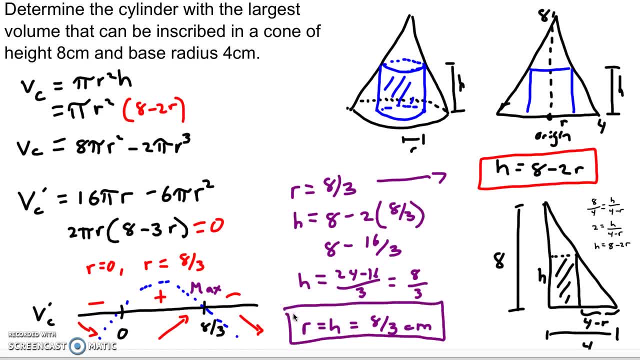 You always want to pay attention to units. They are important. So this is the problem, And again it follows the same essential process as all of these optimization problems: You need to figure out what the function you're looking to optimize is In this case, that's this volume function.